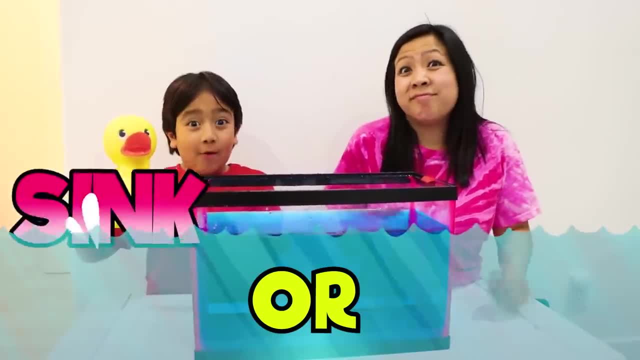 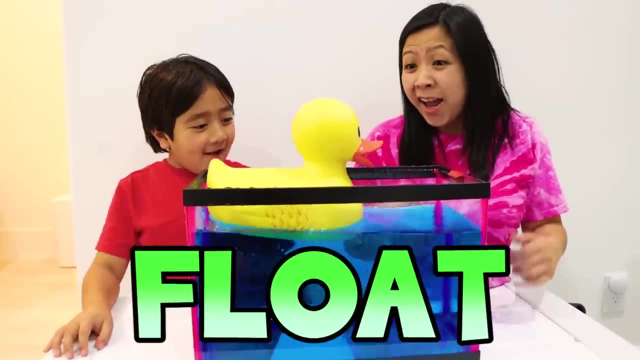 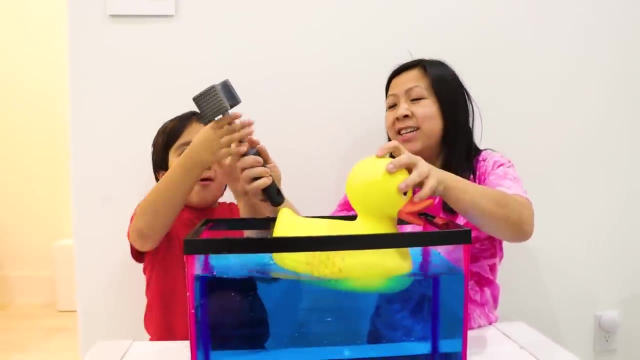 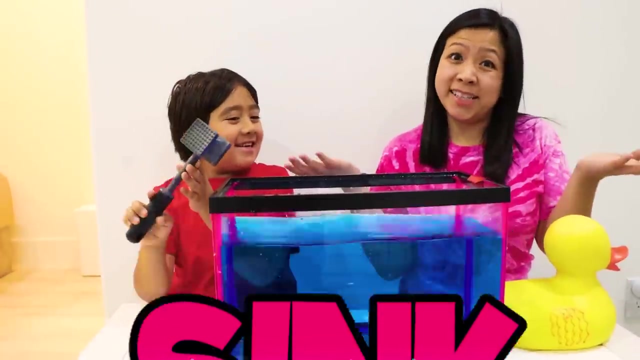 Hey guys, do you think this rubber ducky is gonna sink or float? I think it's gonna float. Whoa, it's floating. Good job, Ryan. Now what about this mallet? Do you think it's going to sink or float? I think it's going to sink. Let's see. 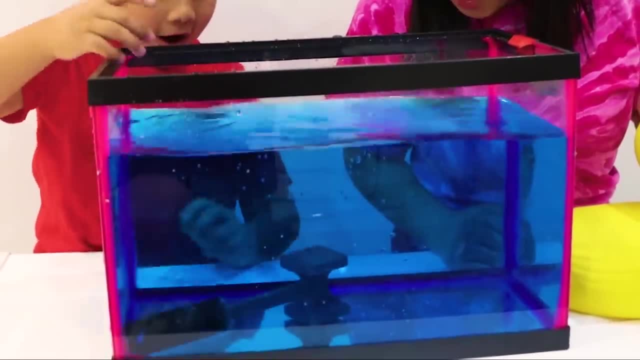 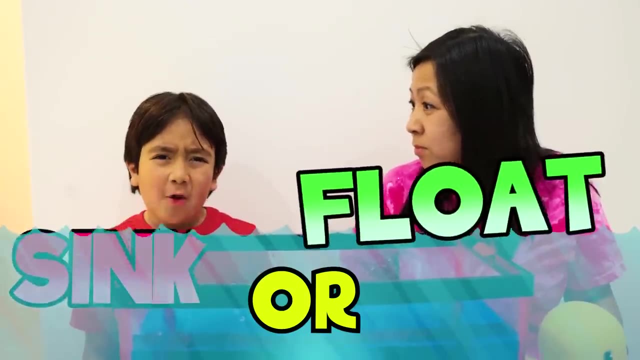 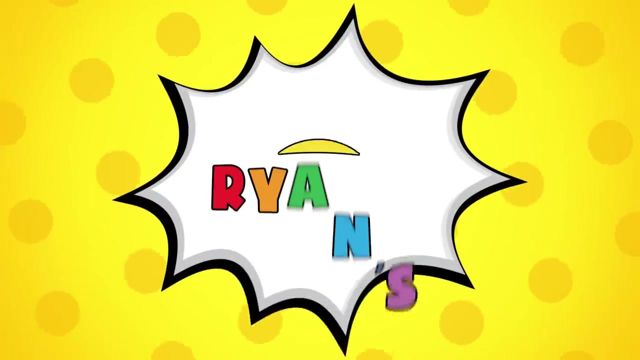 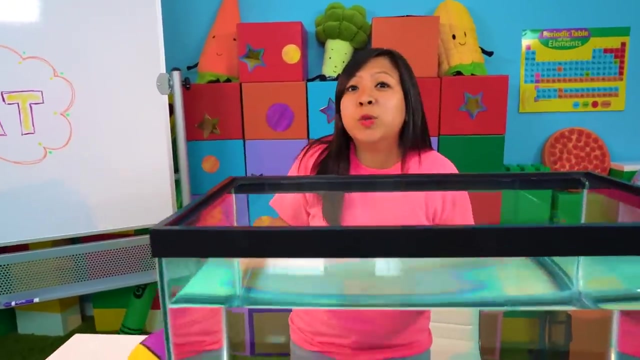 It's sink. Good job. But, mommy, why do you think sink or float? Good question, Ryan, I'll show you. Come on, guys, Where'd mommy go. Welcome to Ryan's world. Did you know an object's ability to sink or float is called buoyancy? But 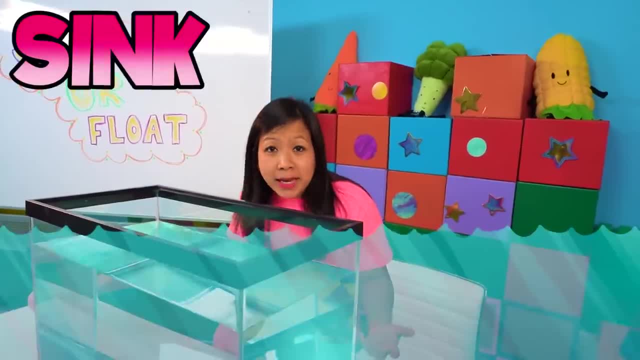 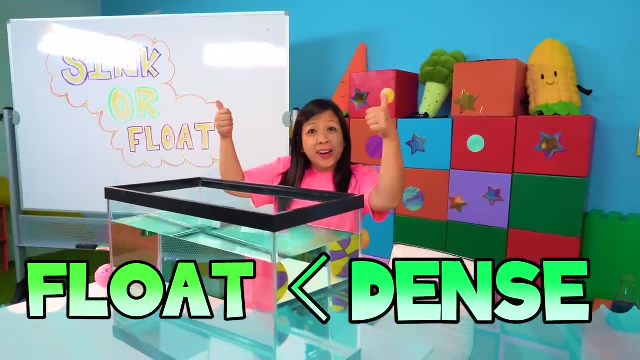 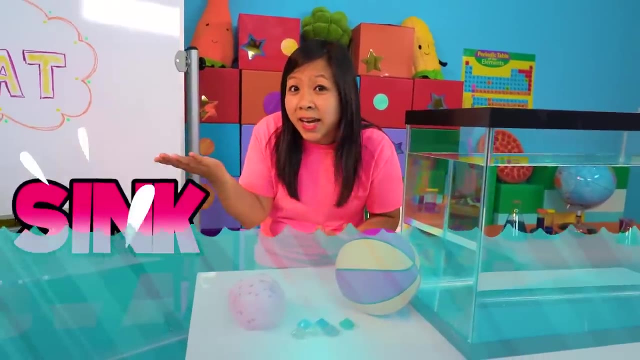 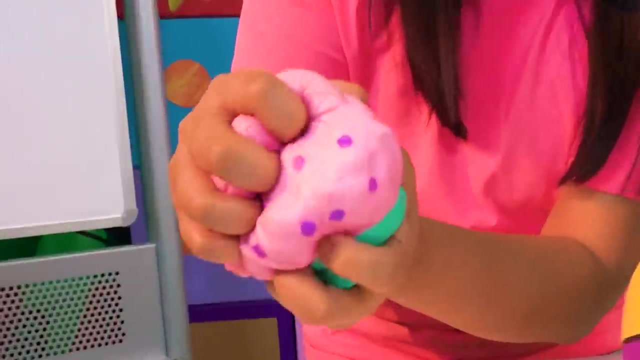 why does an object sink or float? An object will sink if they're more dense than water. An object will float if they're less dense than water. So let's try putting these objects in water to see which one will sink and which one will float. Let's see what we have here: Squishy some diamond jewels and a basketball. 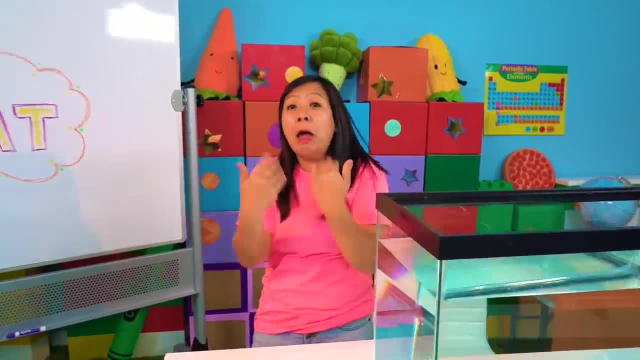 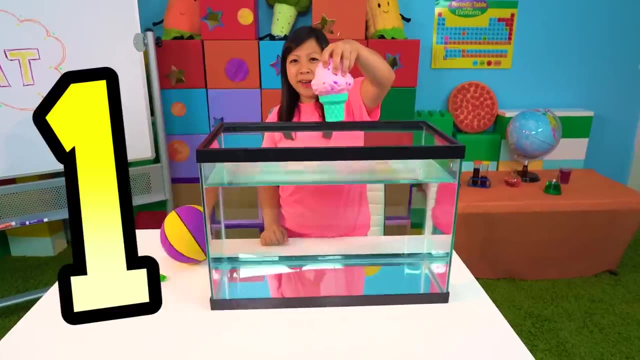 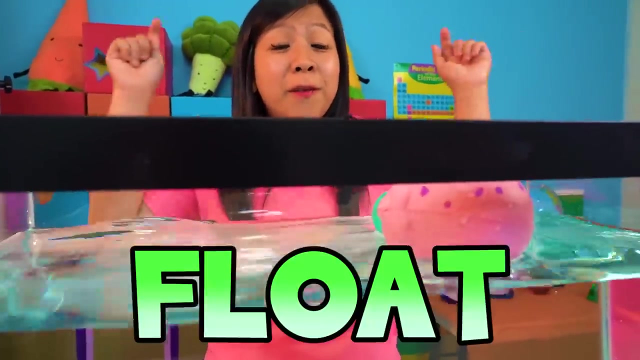 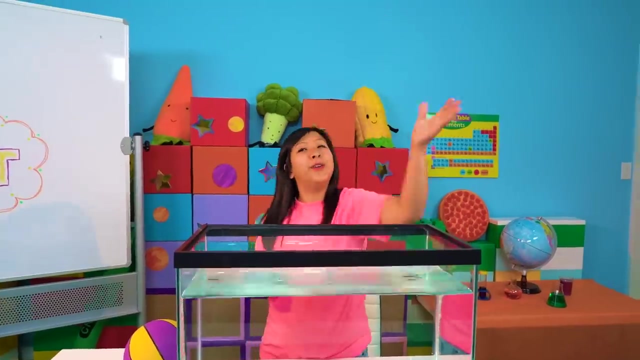 Here we go. Oh, I should get that back. Come back. This squishy toy feels light, but let's see if it'll float in water. All right, One, two, three, Wow, The squishy toy float in water. So what does that mean? It's less dense than water, Yay. 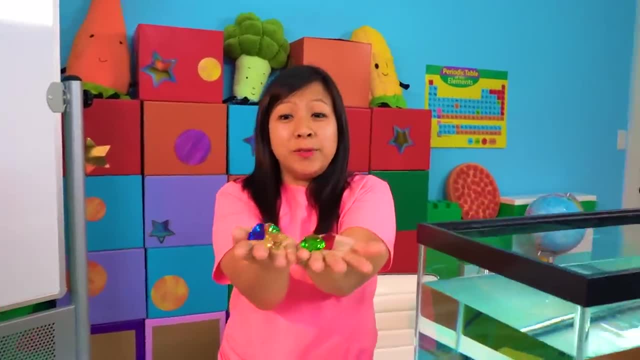 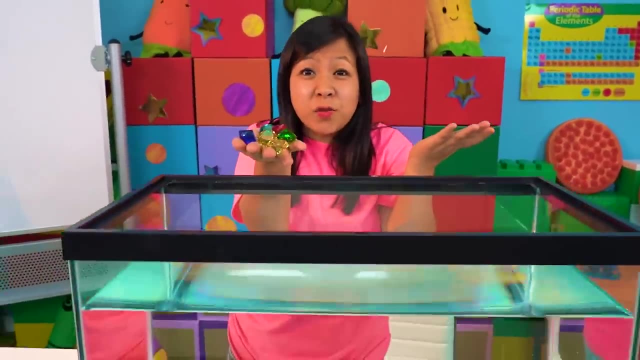 Okay, let's see what we have next. Next we have these stones: colorful, Woohoo, Ah, so bright. They're smaller than the squishy toys. Do you guys think it'll float in water? But they're heavier. Does that make a difference? Let's see One, two, three. 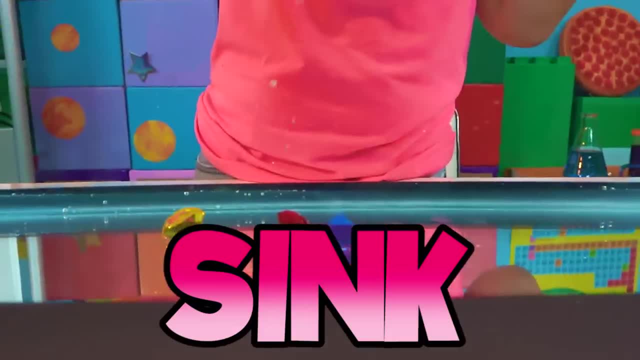 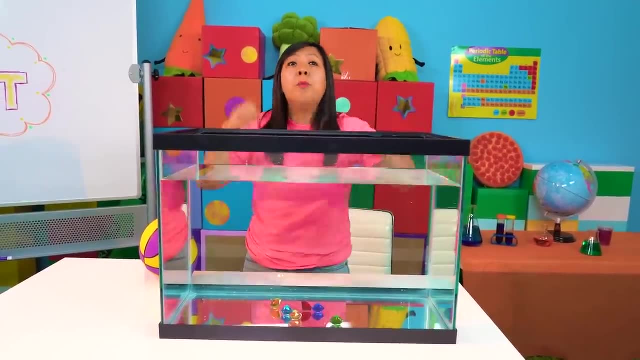 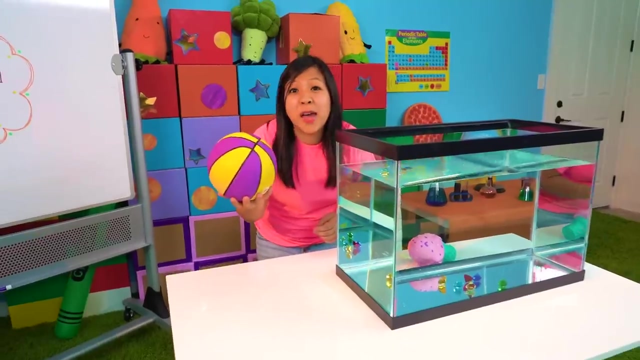 Oh, no, Wow. So what does this mean? These stones are more dense than water. Look, they sink all the way to the bottom. Next we have a basketball. Look it bounces. It's heavier than the squishy. 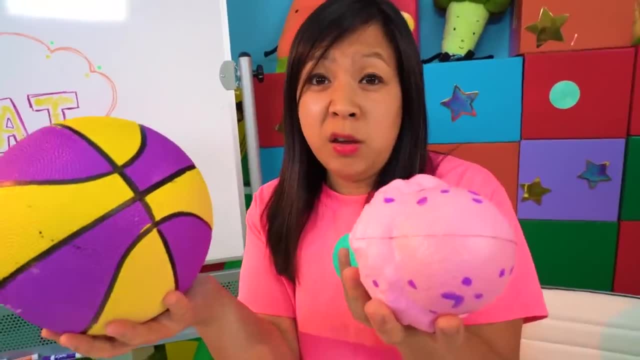 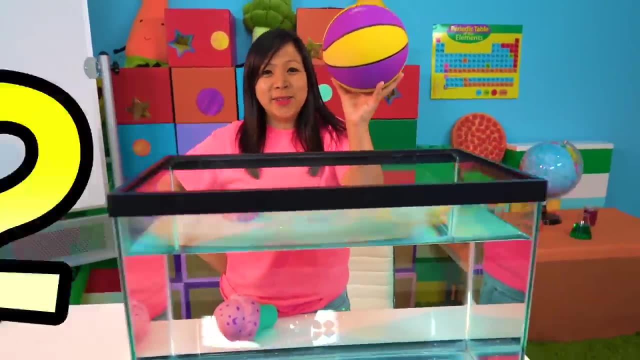 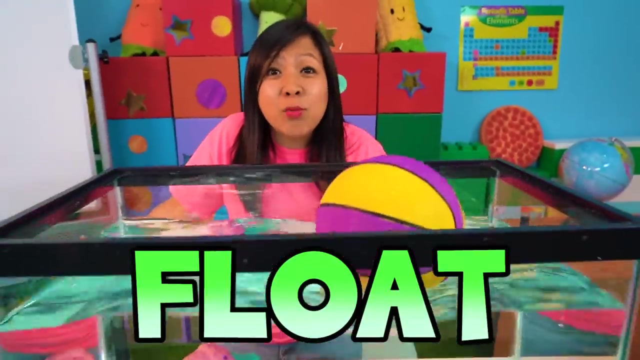 toy. It is bigger than the squishy toy. Do you guys think this will float or sink in water? All right, let's test it out. One, two, three, Whoa. What did you guys notice? It floats in water. 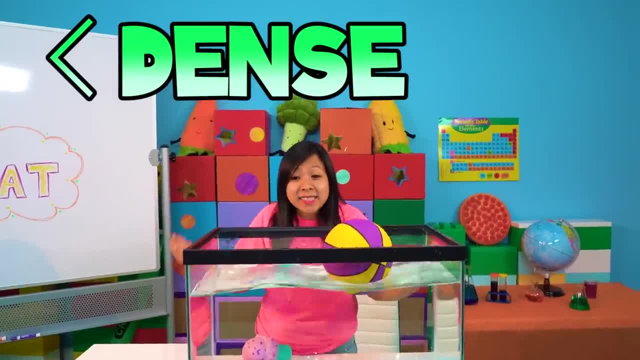 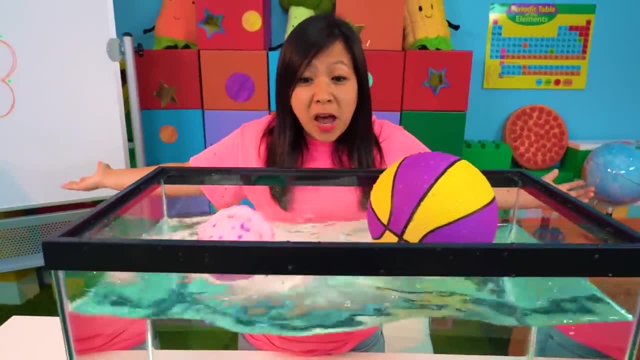 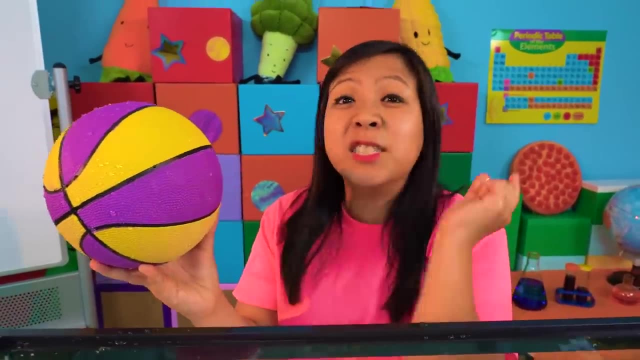 What does that mean? It's less Dense than water, Even though it's bigger and heavier than the squishy toy. They both float. So why does the basketball float? Well, it's hollow and empty inside and it's full of air. 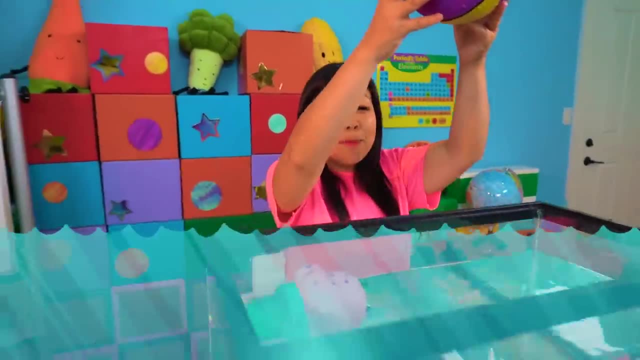 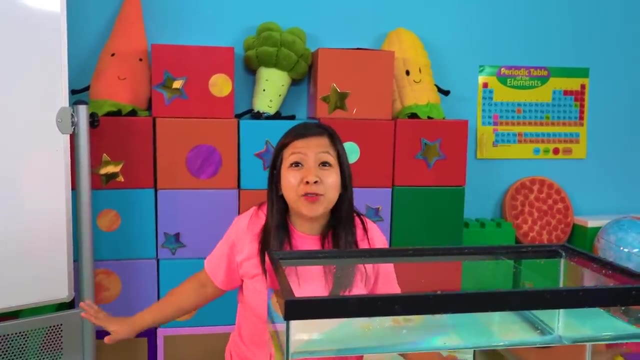 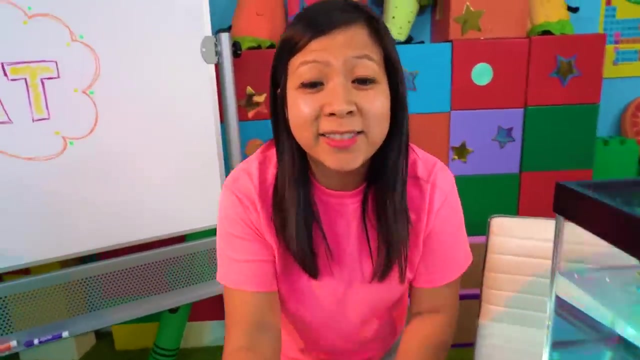 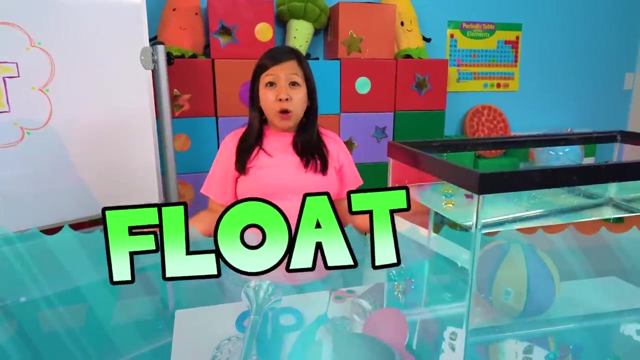 And air is less dense than water, so it helps the basketball float. Woohoo, I have an idea. Let's go grab a whole bunch of other stuff to try. Be right back, Okay, guys, A whole bunch of stuff for us to try, okay. So remember, an object will sink if the density is greater than water and an object will float if the density is less than water. 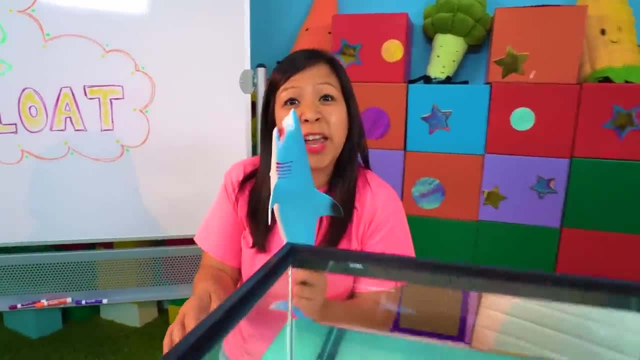 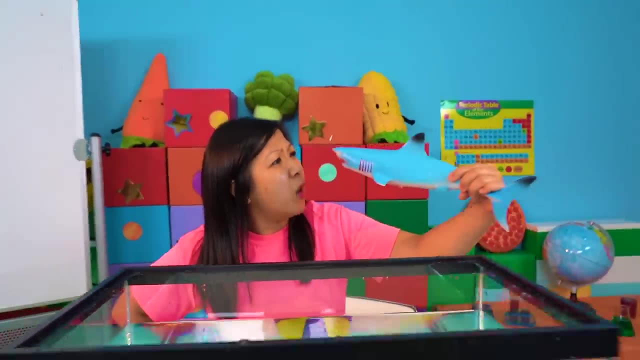 So let's see, Mr Shark, do you want to give it a try? It's not a real shark, It's a toy shark. Sink or float, Let's see. Are you greater than water for density or less? One, two, three. 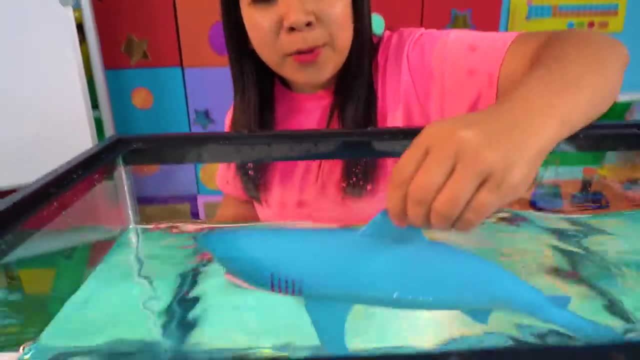 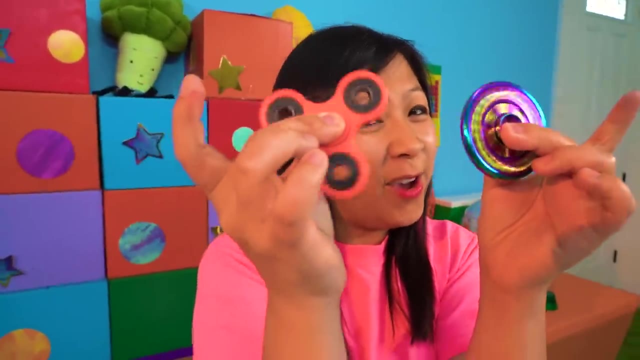 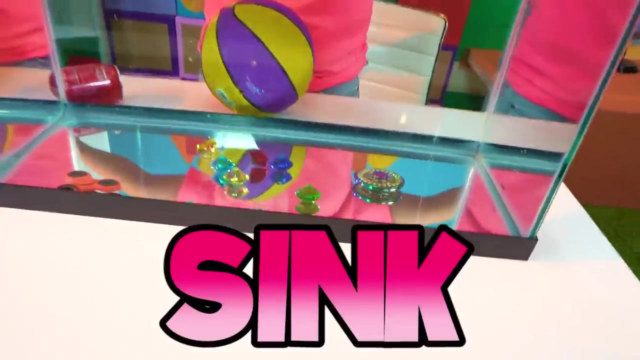 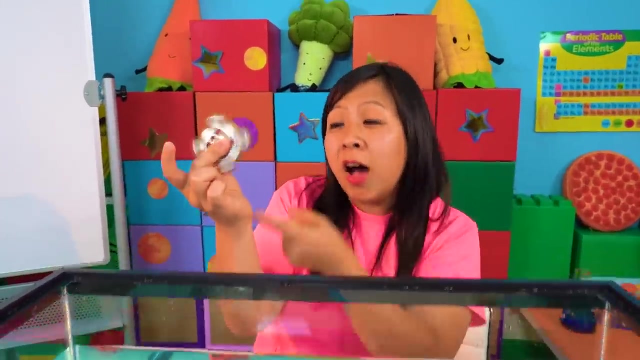 The shark floats. Wow, It must have a lot of air inside. Do you guys remember? these Fidget spinners Sink or float. Let's test it out: One, two, three, They sink. So what does that mean? The density of fidget spinner is greater than water. 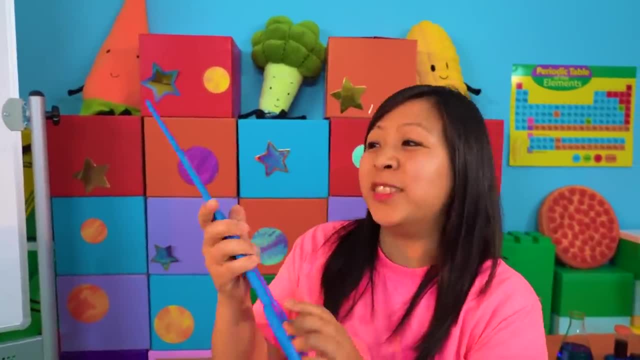 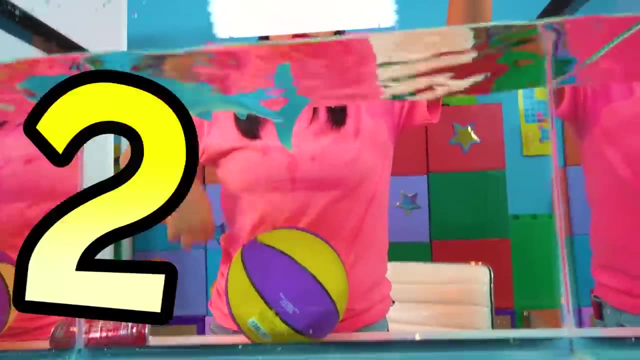 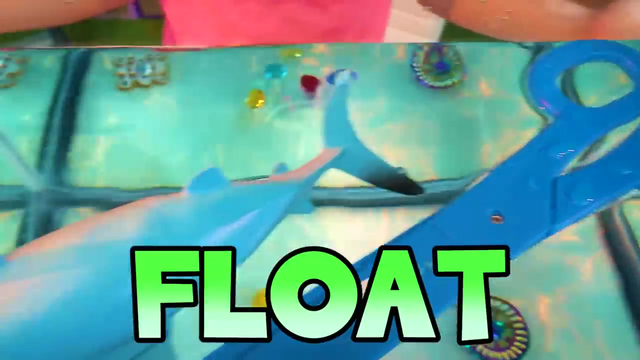 Next, Next Scissors. So this is a plastic scissor, but we're going to see if it sinks or float in water. Are you ready? One, two, three. It floats. Did you guys guess that right? So these are less dense than water, okay. 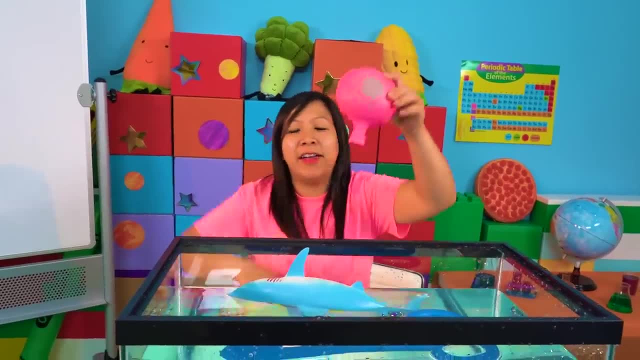 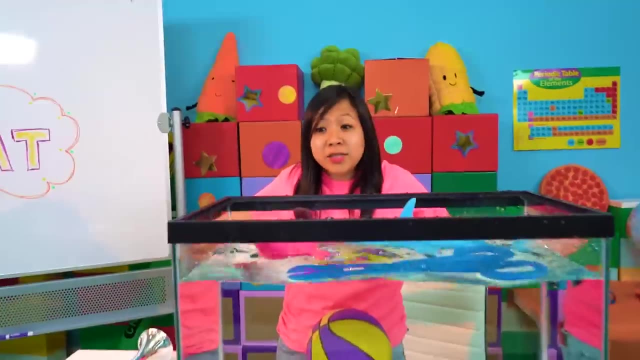 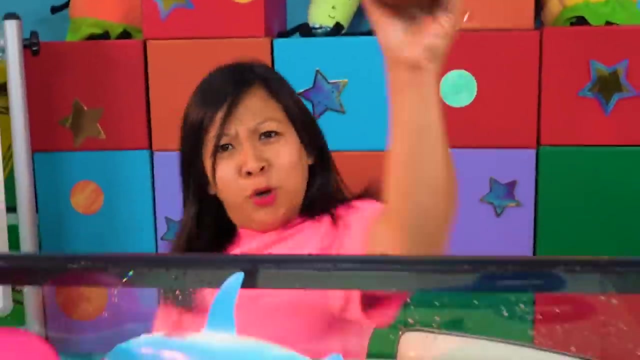 Goofy cushion. Okay, All right, Sink or float, What do you guys think? One, two, three. یہ Who likes to play American football? Hot, hot, Pinker flow. One, two, three. 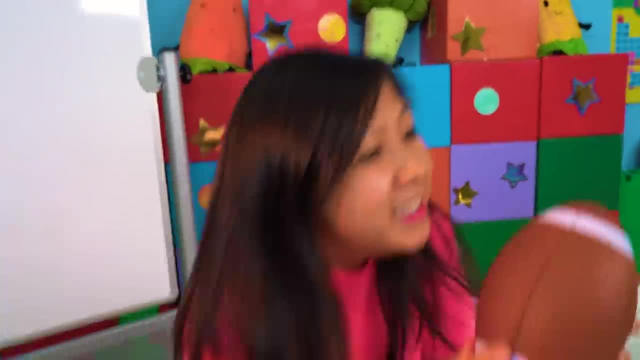 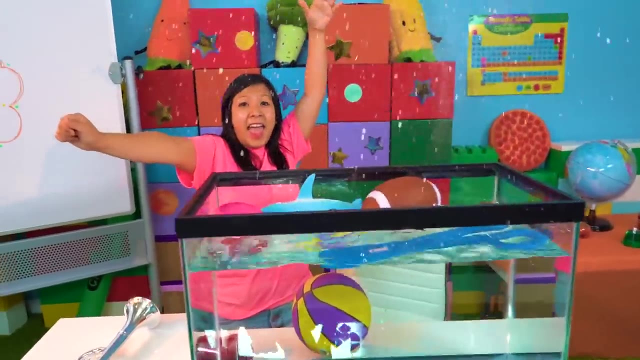 Sorry, I'll be right back. Obviously, No, not good at American football. One, two, three Hot hot catch, Yay, Awesome Flows. Wow, So far we're doing great, We're getting there. 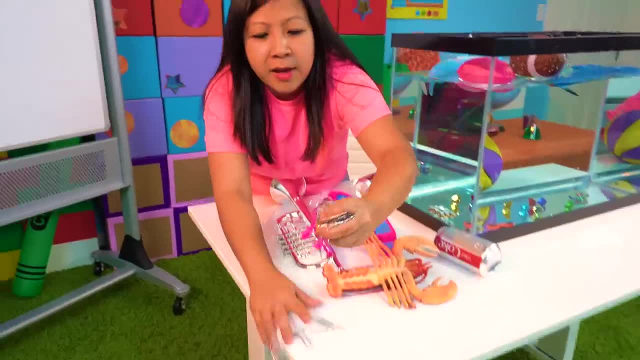 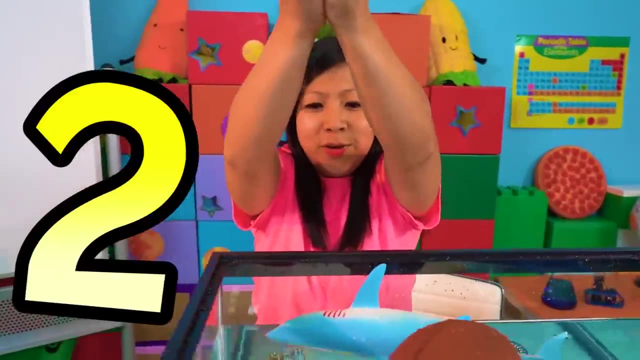 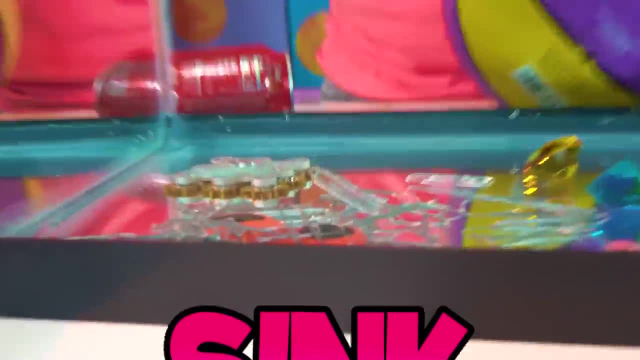 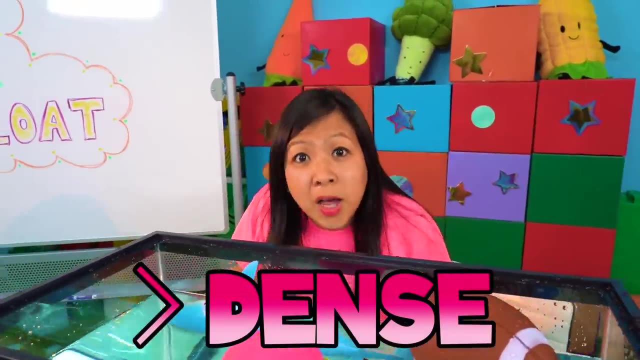 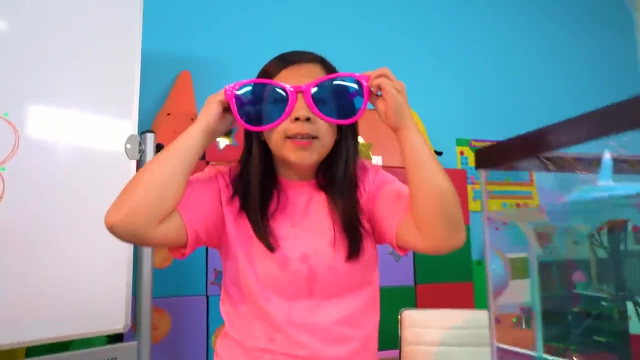 So what's happening? They all sink. That means the paper clips density is greater than water. Okay, what's next? This is so fun. What about the giant glasses? These sink, or float, Any guesses? All right, bye-bye glasses. 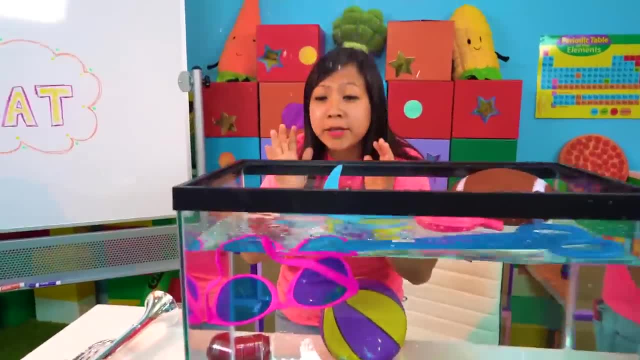 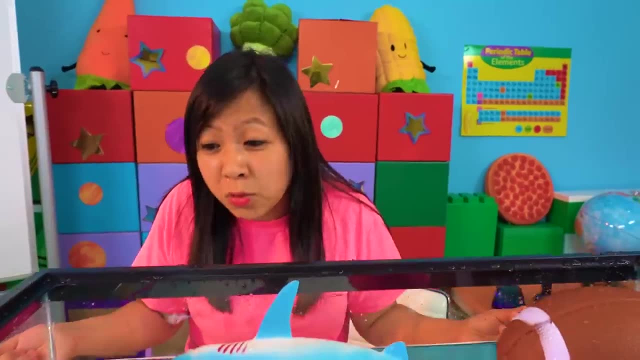 One, two, three. Is it gonna sink or is it gonna float? It's hovering. it's hovering. What do you guys think? I think it's pretty close to water's density. That's why it's right there in between sinking and floating. 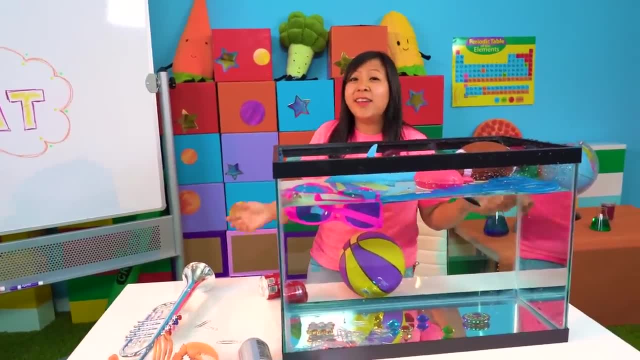 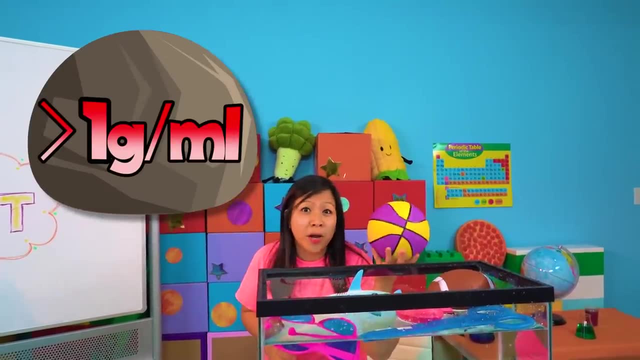 So since you guys didn't ask what is the density of water, It is. the density of water is one gram per milliliter, So anytime an object's density is greater than one gram per milliliter, it sinks. Anytime an object's density is less, 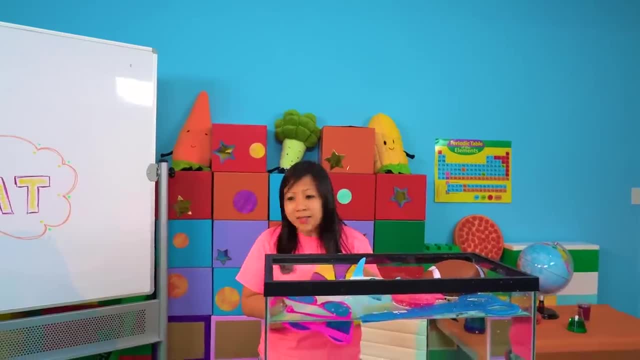 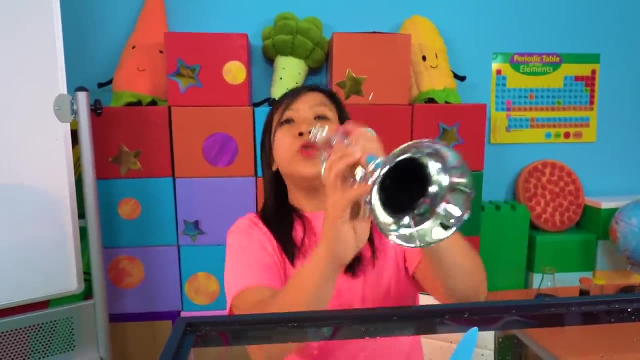 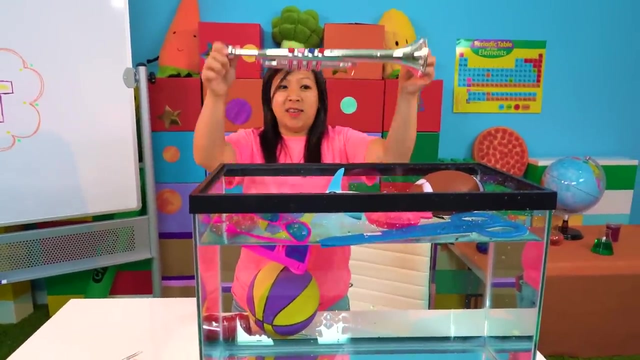 than one grams per milliliter. it floats. Um what else? Trumpet, Sink or float, Don't forget, there's lots of air inside here, lots of holes. It is pretty flat, Plastic-y. One, two, three. 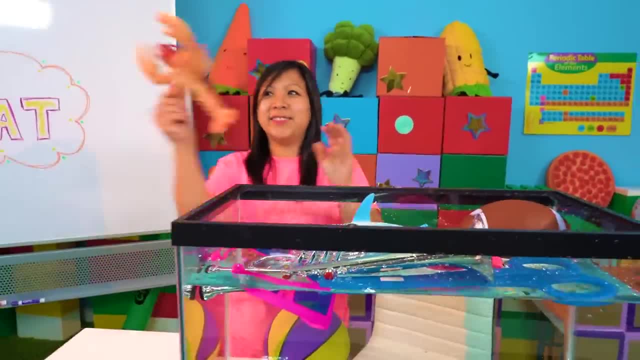 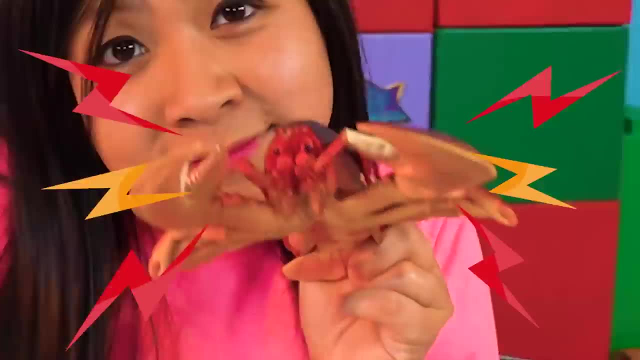 Float. All right, Lobster, you guys like lobster? Hey, Mr Lobster, do you sink or float in water? Well, I am a lobster, so I think I'm going to sink. Oh okay, Let's see if it's true. 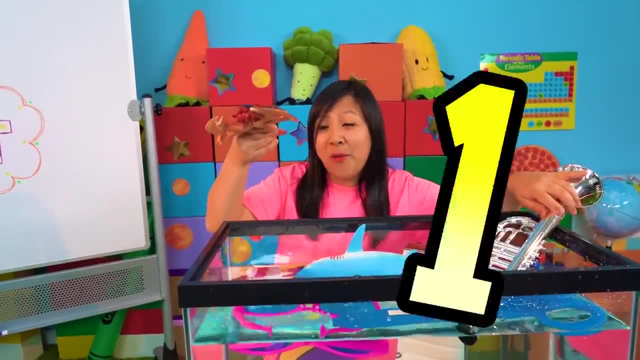 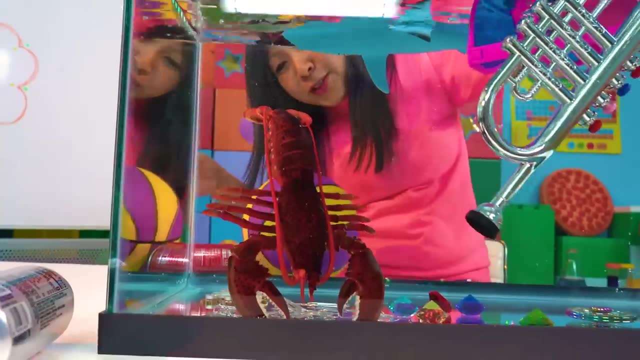 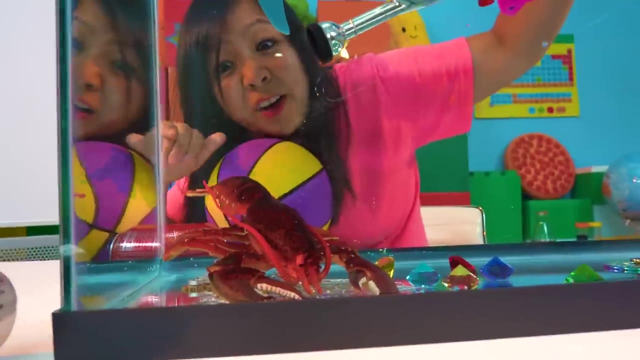 He thinks he's gonna sink. What do you guys think? One, two, three, Oh Oh, Mr Lobster did sink. Bye-bye lobster. Good thing he likes water, huh. So what does that mean? Density is greater than water. 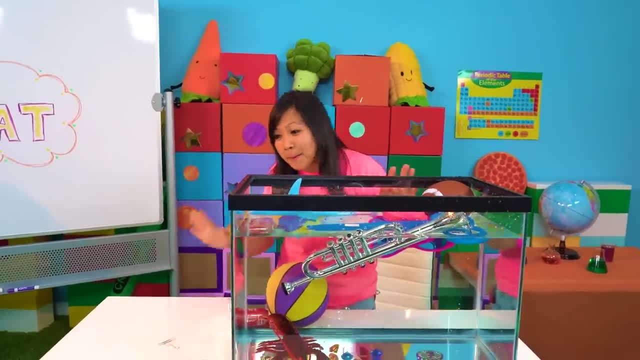 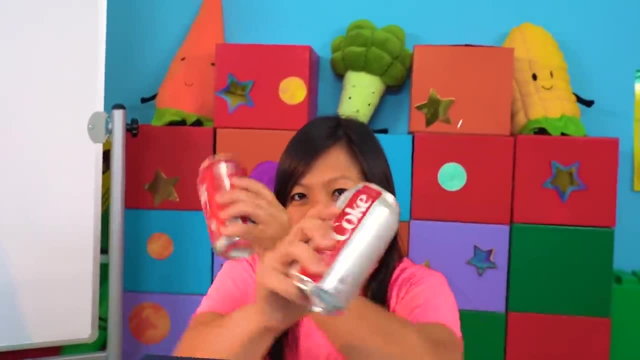 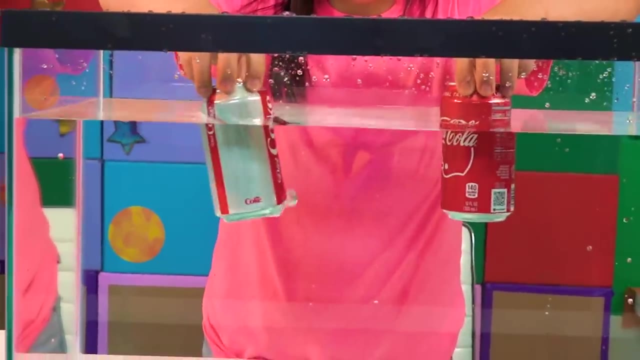 Okay, we're gonna clear out the tank because I have a super fun experiment: Diet Coke versus regular Coke- Which one will sink and which one will stay afloat? All right, let's put it into the water. Okay, guys, we have to wait, okay. 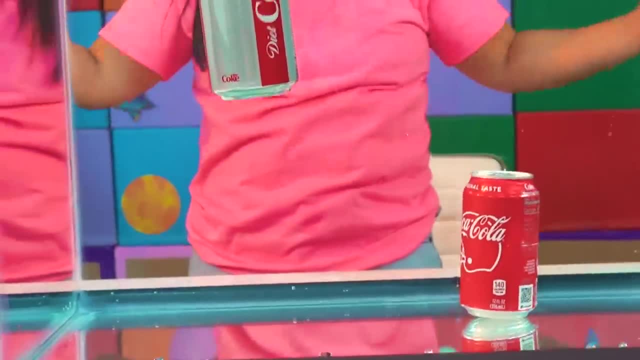 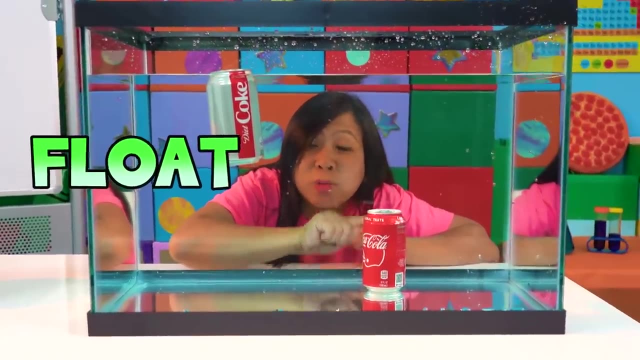 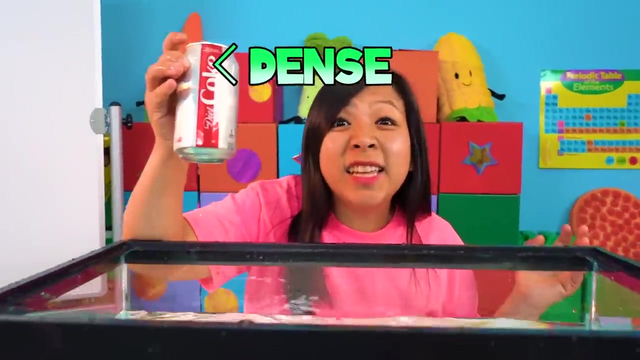 Something cool is gonna happen. Wow, look what you guys noticed: That Diet Coke float and that regular Coke sink. So what does this mean? The Diet Coke is less dense than water, but the regular Coke? Oh, where are you? Regular Coke? there you are. 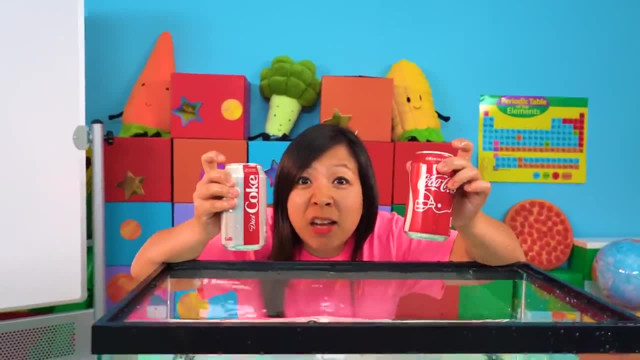 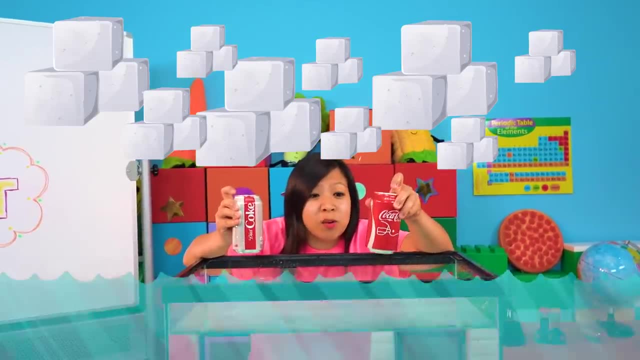 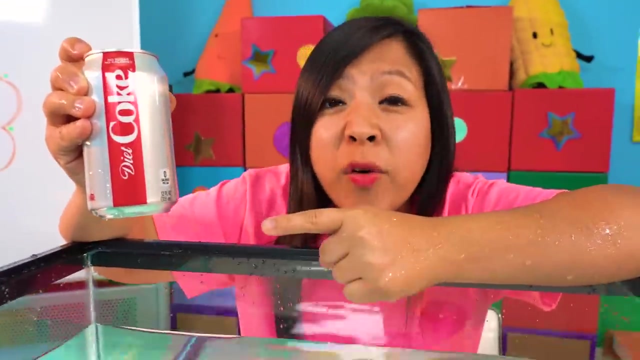 It's more dense than water. Do you know why? Because this actually has lots and lots and lots of sugar inside. So the sugar is more dense than water. so it sink the Coke And the Diet Coke actually has less than one gram of sugar. 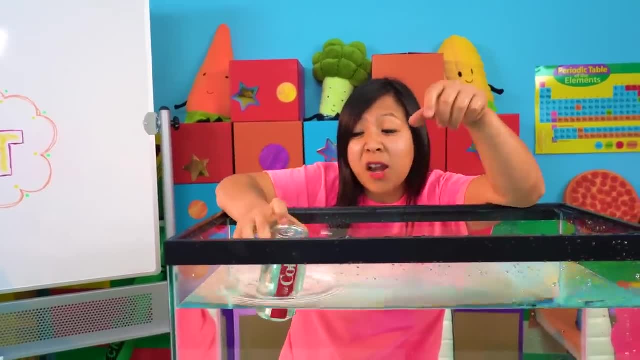 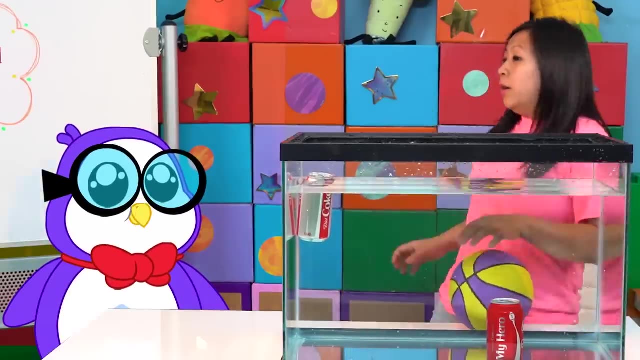 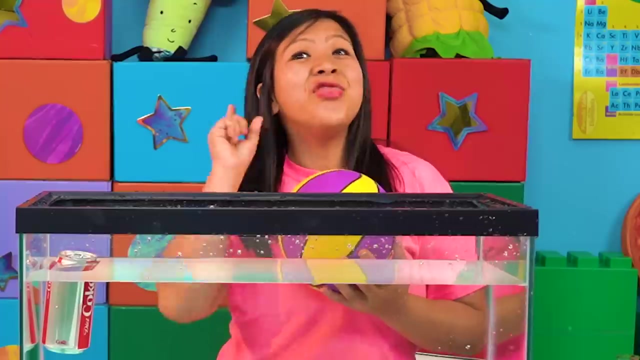 so mostly just water and air inside, so it floats Whoa. Excuse me, Ms Ryan's mom? Yes, Peck, I'm doing some homework on buoyancy and I'm trying to understand how these giant cruise ships are able to float in the ocean. 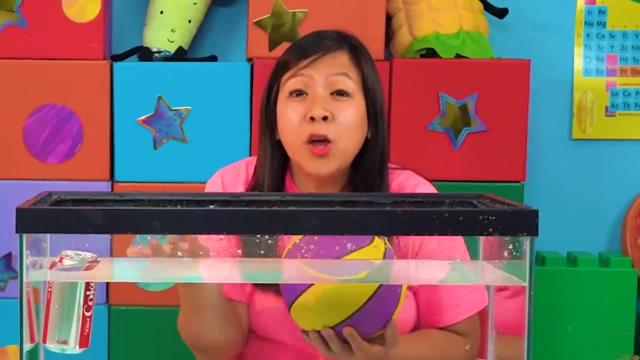 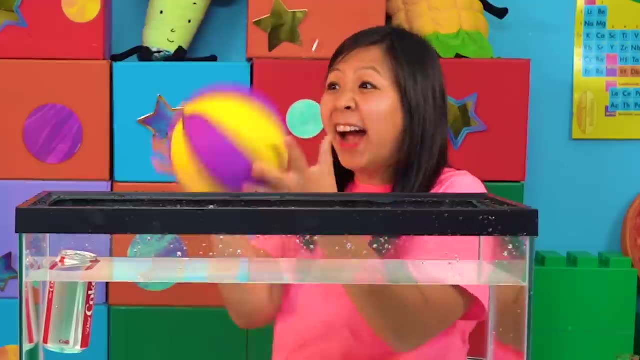 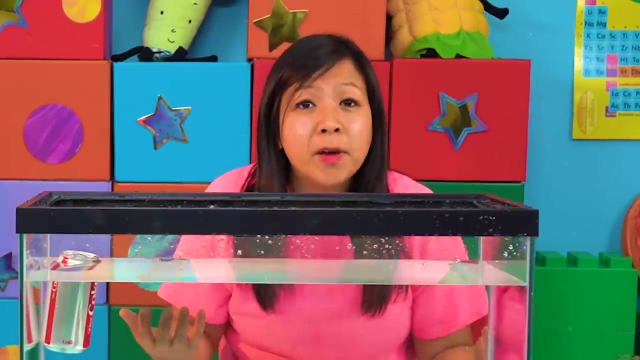 That's a good question. Peck, Those cruise ships can float in water because it's hollow, like this basketball, and full of air. It's hollow and full of air, Got it. But that's not all. Peck, It's because also the shape of the cruise ship. 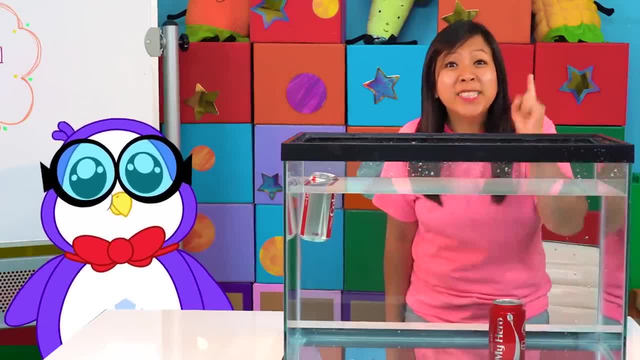 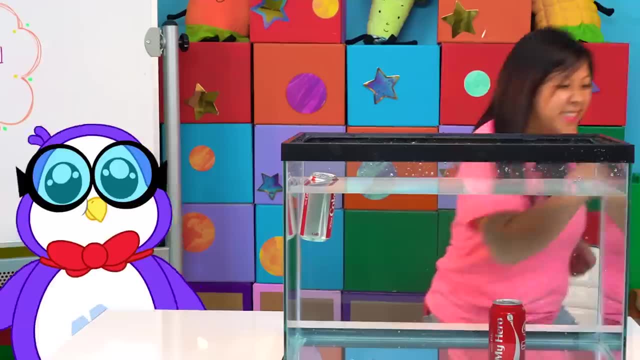 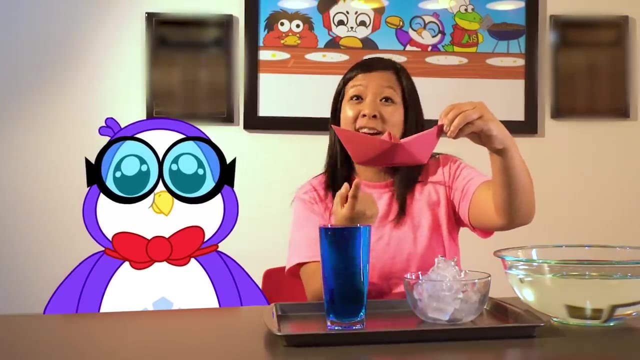 I have an idea. Let's do one more experiment. Oh joy, Another experiment. I love experiments, Let's go. Did you know that ship is shaped so that most of it is above water? That way it doesn't displace too much water. 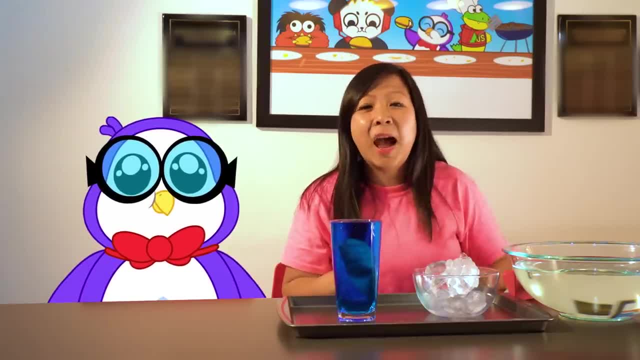 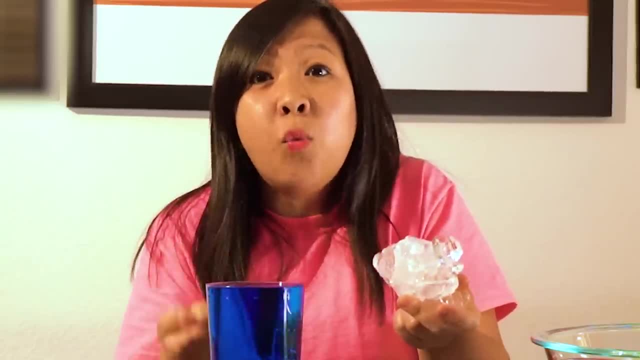 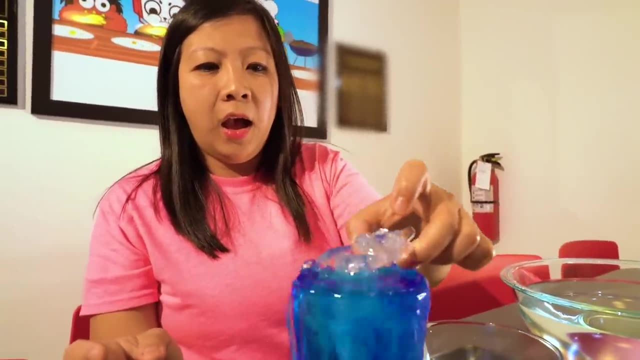 Displace. Yeah, Let's try this. I'm going to put ice- oh it's cold- In this cup that is full of water and see what happens. You guys ready? Oh, it's so cold, Okay, Whoa. 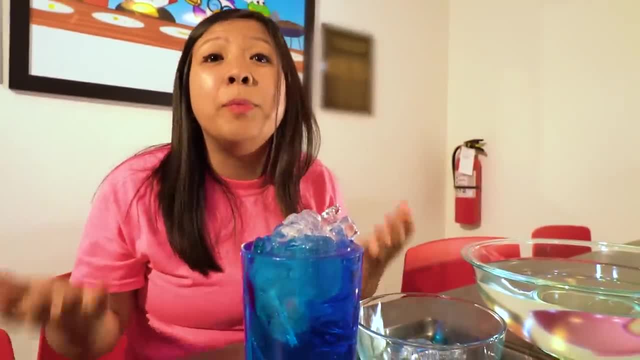 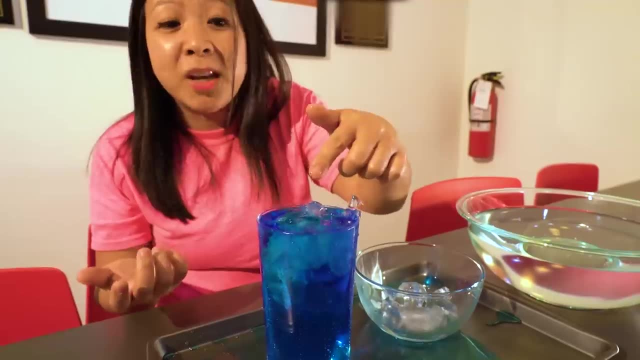 Whoa, The water spilled everywhere. Yeah, so when we put the ice in a cup of water that's already filled, the water spills out, right. So when an object pushes water out of the way, this is called displacement, Yeah. 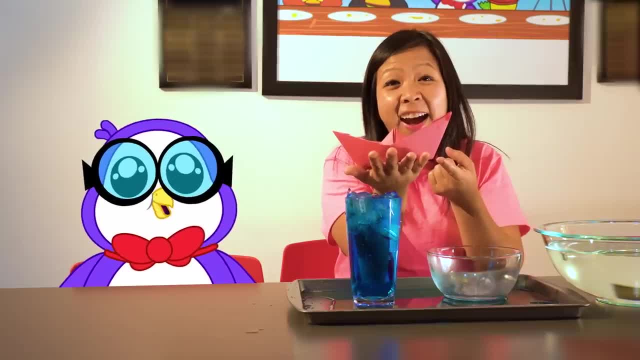 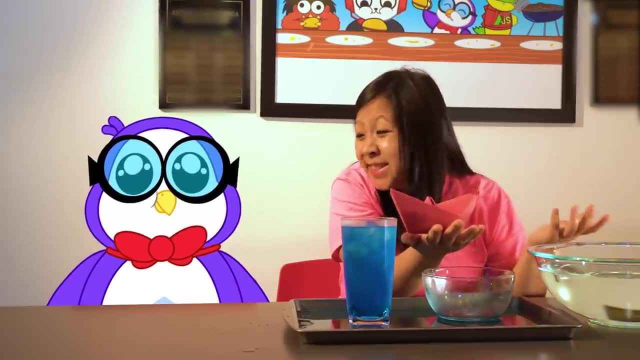 This is why ship don't sink. They are hollow like the basketball and full of air, and they're shaped so that they don't displace too much water. That's right. Oh joy, I can finish my homework now. Thank you, Ms Ryan's mom. 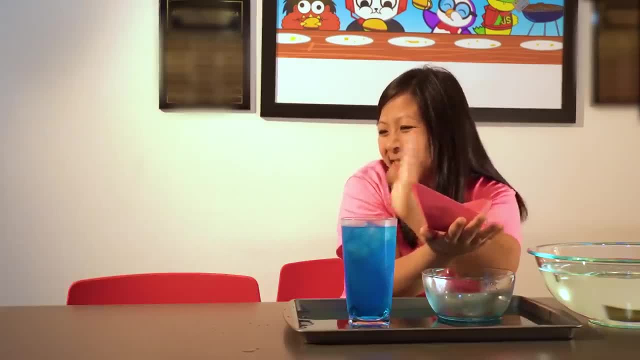 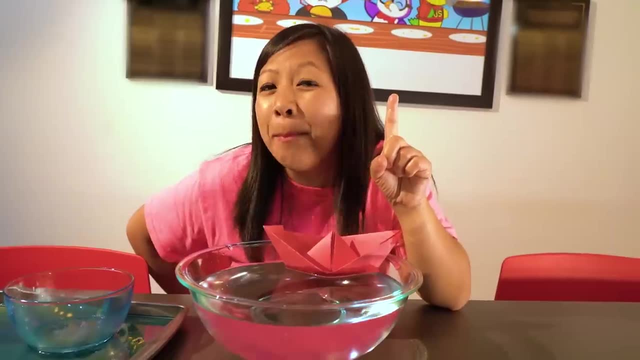 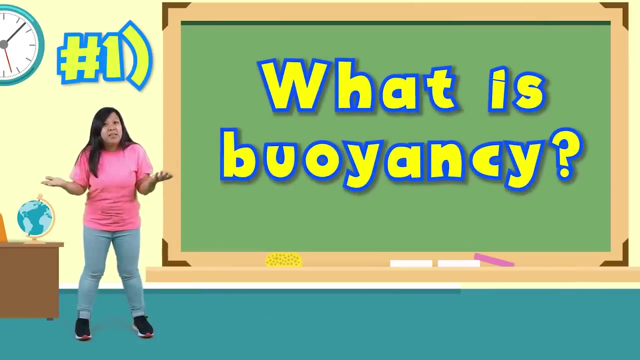 See you later. You're welcome, Peck Bye. So I think that now we're an expert on objects sinking or floating in water. Let's try a pop quiz. Let's go Question number one: What is buoyancy? Is it A an object's ability to sink or float? 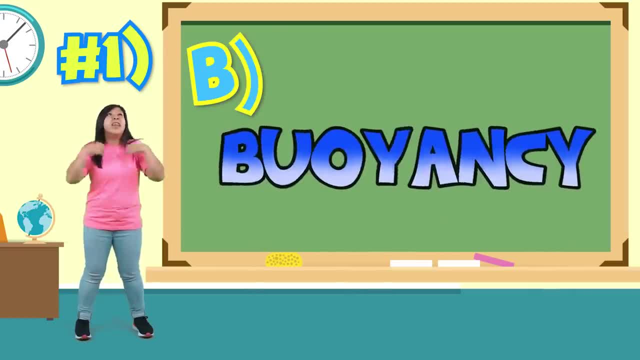 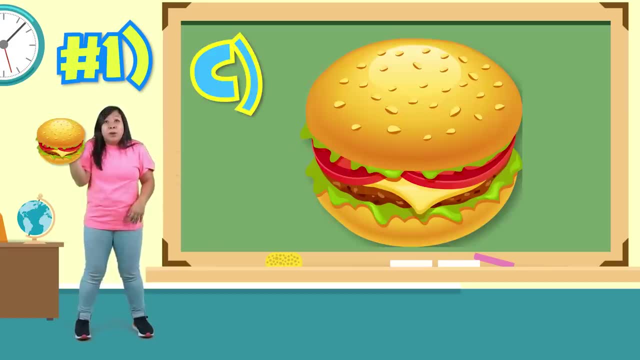 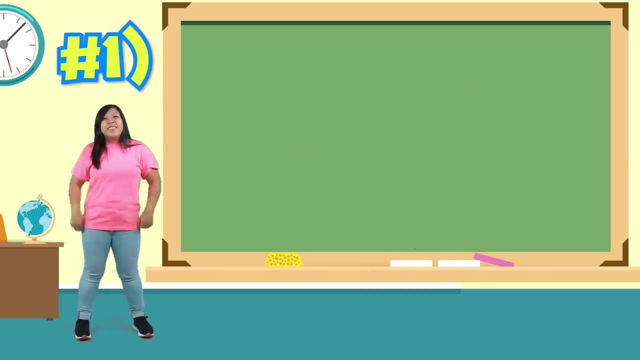 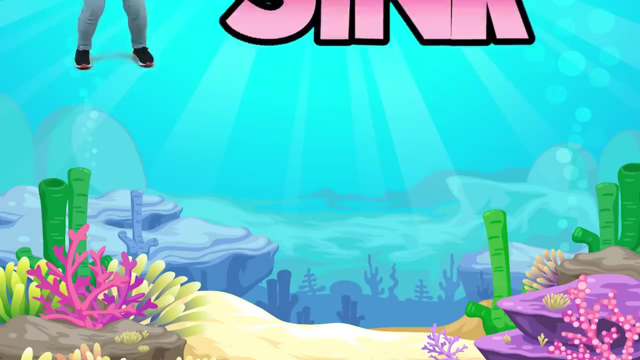 Or is it B? buoyancy is a buoyant hook Or is it C? is buoyancy a cheeseburger? B- Any guesses? The answer is A. Buoyancy is an object's ability to sink float or float. 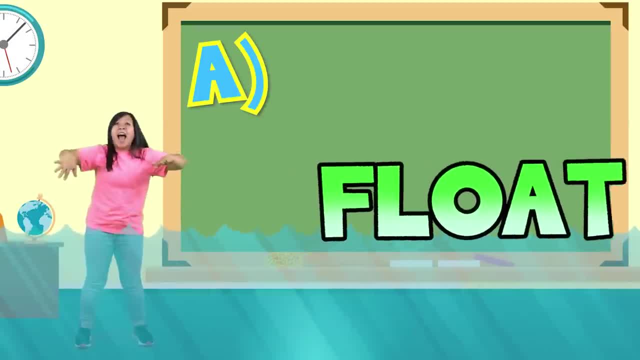 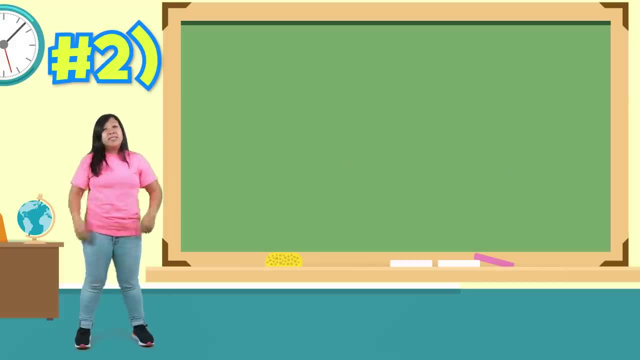 Yay, All right guys. Let's move on to question number two. Why does object sink? Is it because A- they're blue, All objects that's blue float. Or is it B- they like to swim. Or is it C- they like to swim? 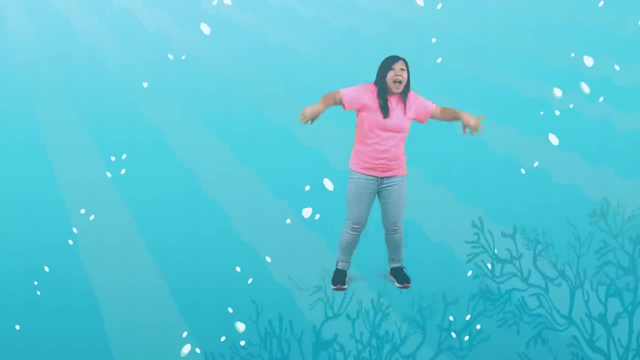 Or is it D? they like to swim? Or is it C? they like to swim? Or is it D? they like to swim? Or is it C? they are more dense than water? Or is it D? they are more dense than water? 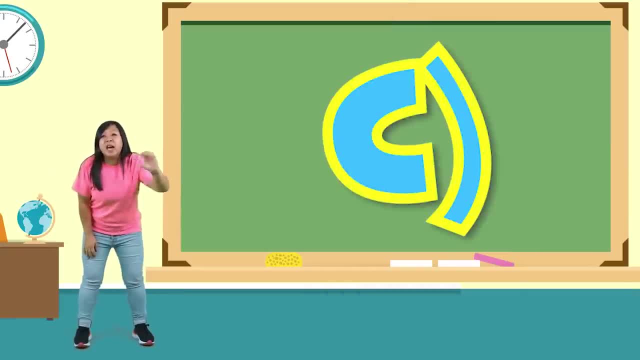 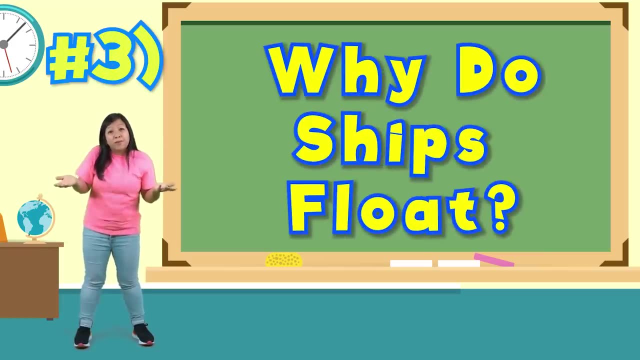 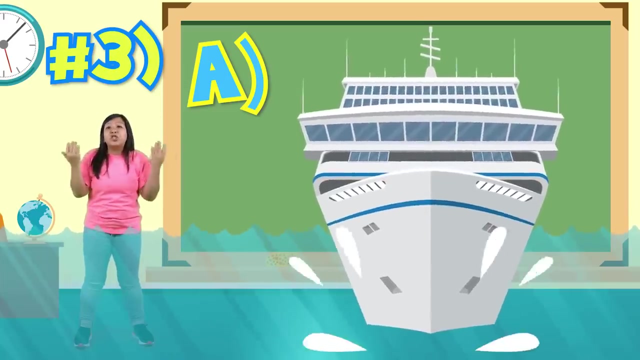 So what's the answer? Why do objects sink? It's because, C- they are more dense than water. Question number three: Why do ships float? Is it because- A- they're hollow full of air and their shape doesn't replace too much water? 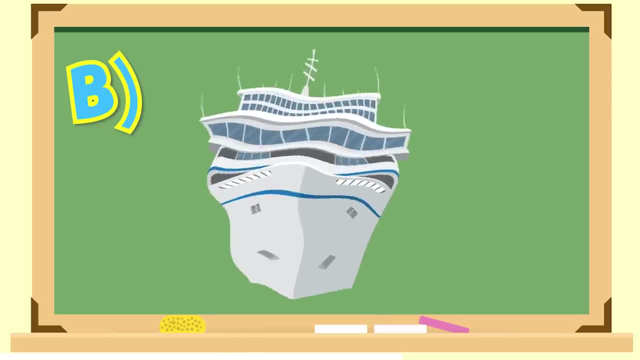 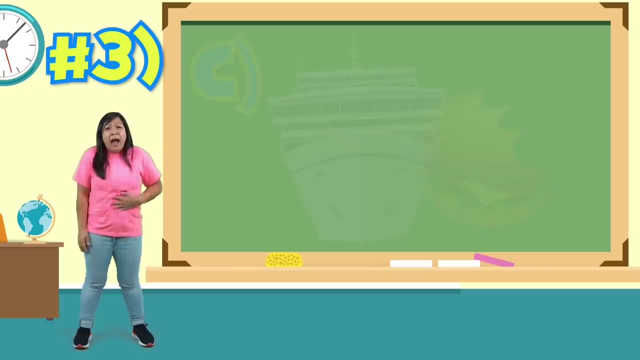 Or is it because B they're hollow full of air and their shape doesn't replace too much water? Or is it because B they're made of squishy fruit? Or is it because of C, they're hungry? Do you know the answer?